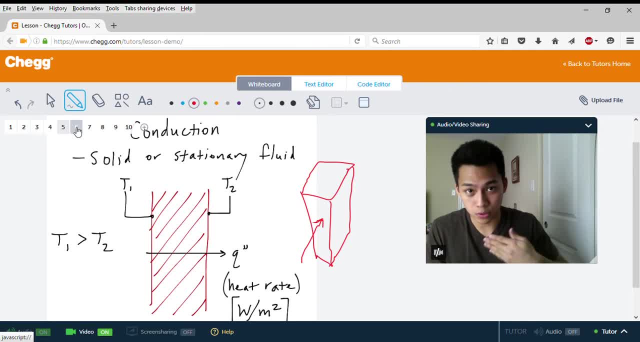 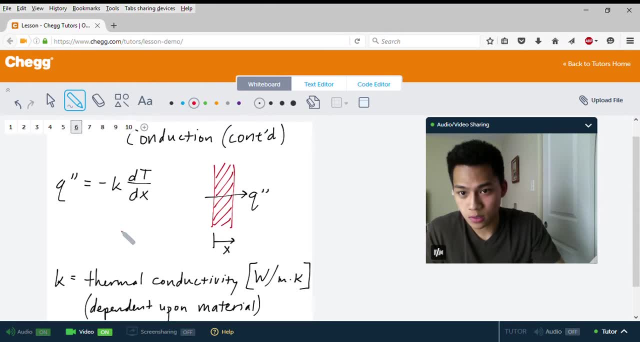 than the other. The heat from that hotter side would transfer through the solid object. So that's the equation for conduction. We have Q double prime, which is the heat rate is equal to negative K times dT over dx, which is essentially the change in temperature, with 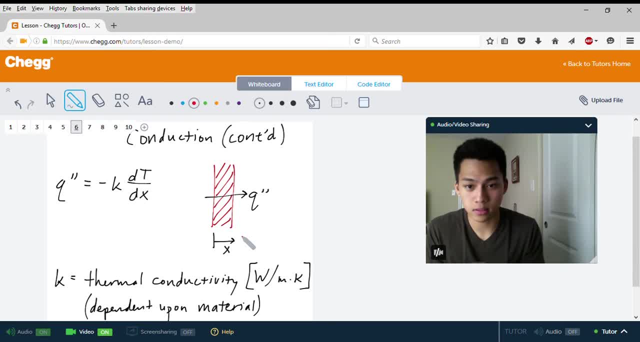 respect to the change in length. So again, if we have our 2D drawing of a brick here, that x distance is right. here It's from one side to the other that length. And then we also have the heat rate Q. 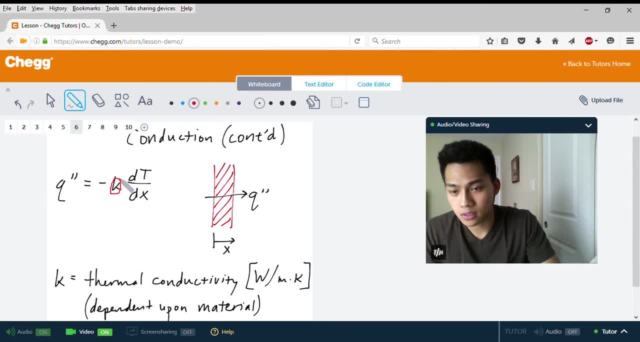 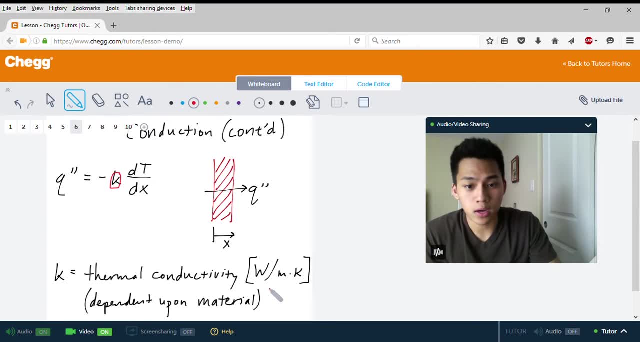 But K is in this equation. Let me circle that. K is essentially the thermal conductivity, It's a coefficient And the unit is watts per meter kelvin And K is dependent upon the material. So the K4 steel is different than the K4,, let's say, some kind of rock. 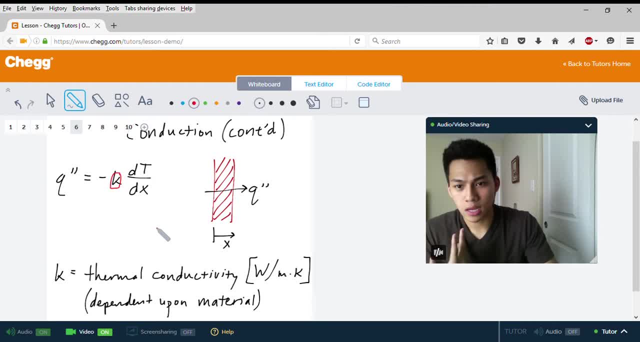 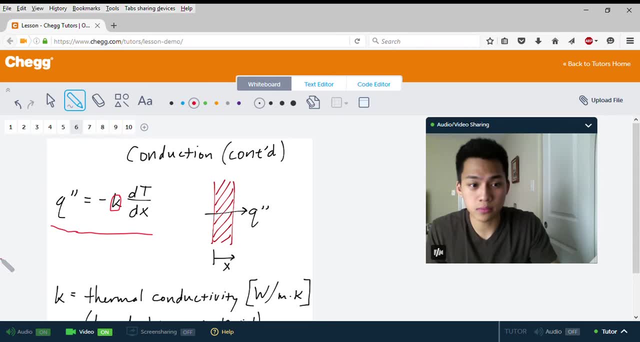 like a brick. So that is pretty much how you solve a conduction problem using this equation. right here, Subtitles by the Amaraorg community. This pretty much governs conduction. The heat rate is equal to negative K times dT over dx. 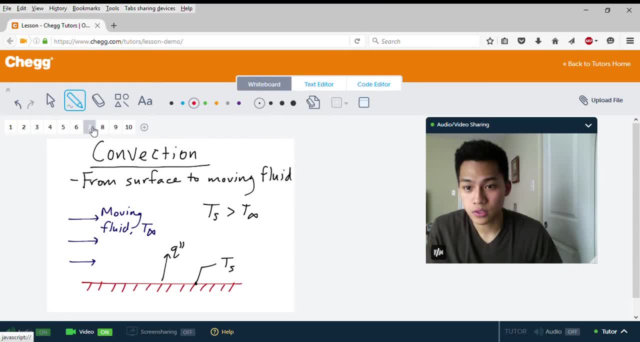 Now the next mode of heat transfer is convection. So what convection is? it happens, the heat transfer happens from the surface to a moving fluid. So as you can see in the drawing here we have a surface- Let's say it's any surface- with moving fluid blowing over the top. So 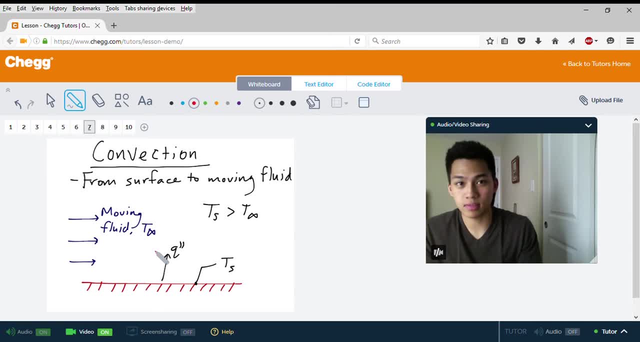 say, for example, you have a heat transfer. Let's say we have a hot, a hot bowl of soup, If the surface of that soup has a certain temperature, a really hot temperature, let's say 100 degrees Fahrenheit, if you blow over. 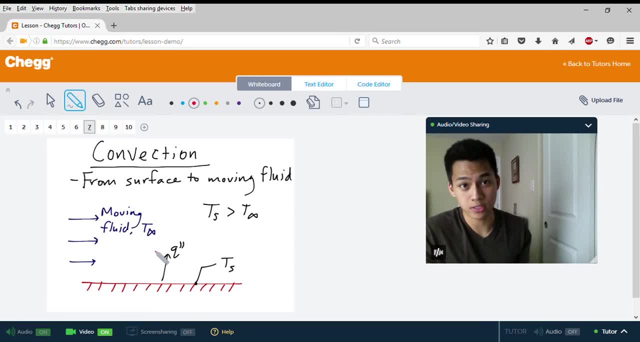 the top of it, you're essentially creating convection. So that's essentially how you cool something. that's hot is by blowing out a fluid, and that fluid is moving. So, as you can see here we have a moving fluid, let's say at a temperature TInfinity. Now for 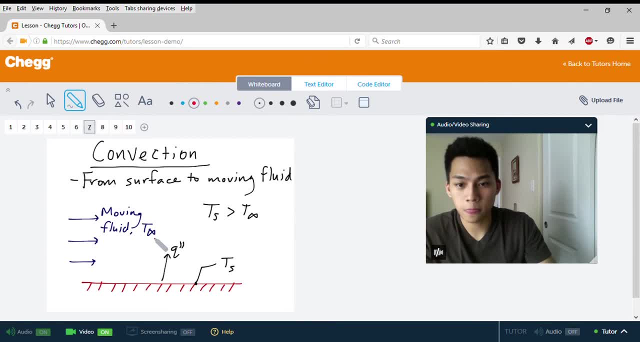 example, you're using the temperature TInfinity And if you blow over the top of it, that's essentially tea and fainting, And if you blow over the top of it, that's essentially a moving temperature T infinity, and we have that surface temperature And in this case, in the same 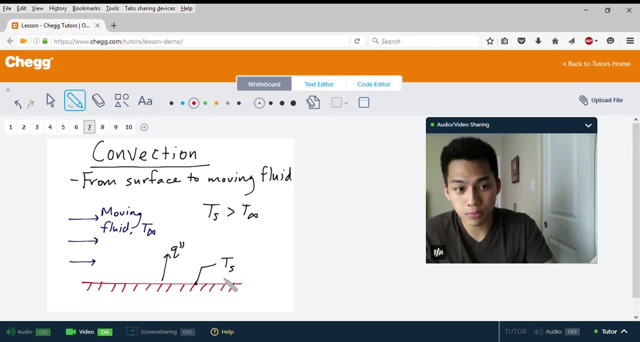 case with a bowl of soup, the surface temperature is greater than the temperature of moving fluid, which means the heat rate would go from the surface to the moving fluid. That means that the amount the heat from the surface is essentially decreasing and it's dissipating. 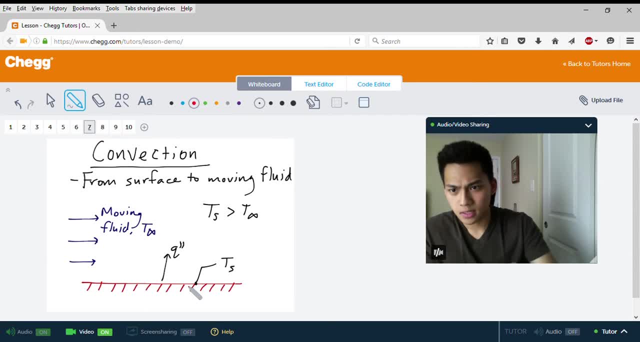 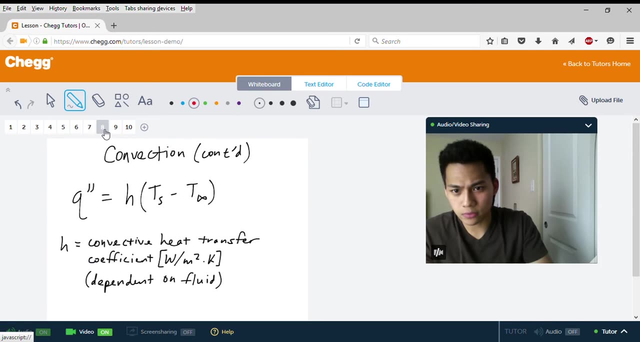 because the fluid is blowing over the top. So again, when you think of convection, you can think of using a fan to cool something or using your own breath to blow onto a surface to cool it. So the equation for convection is Q, double prime, which is the heat rate. 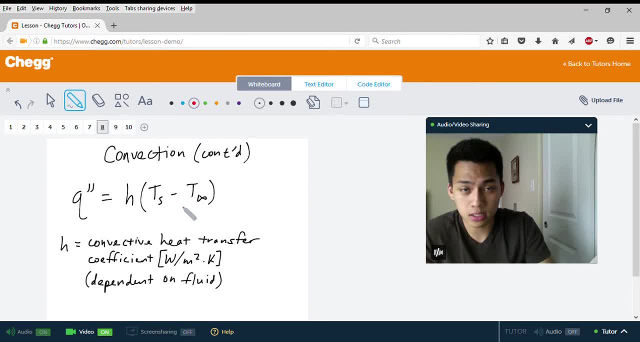 is equal to H times surface temperature minus the temperature of the moving fluid. So we have here: H is the convective heat transfer coefficient, which is in the units of watts per meter squared times Kelvin And again like similar to the thermal conductivity of. 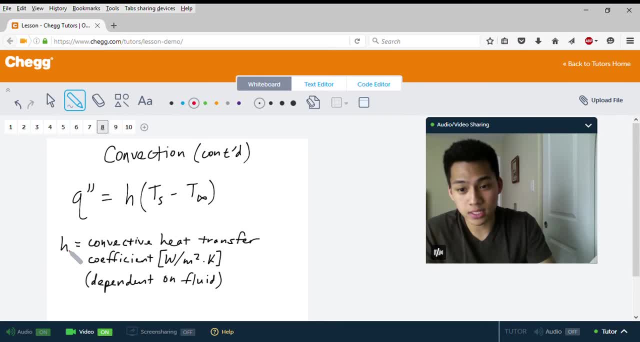 conduction. H is dependent on the fluid that's blowing over whatever surface. So let's say you have H of air is different than H of, let's say, water, Because in some cases of convection, not only can you use air to cool something, but you can use air to cool something. 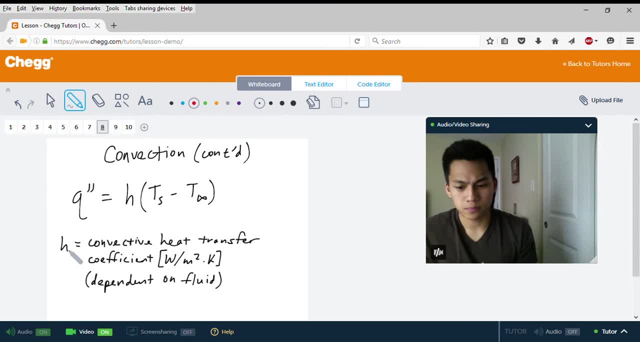 And a lot of machining applications. they use a cooling fluid, They spray it onto the item that's being machined And essentially what's happening is convection. So H is dependent on the fluid. It could be air, water or any other fluid. 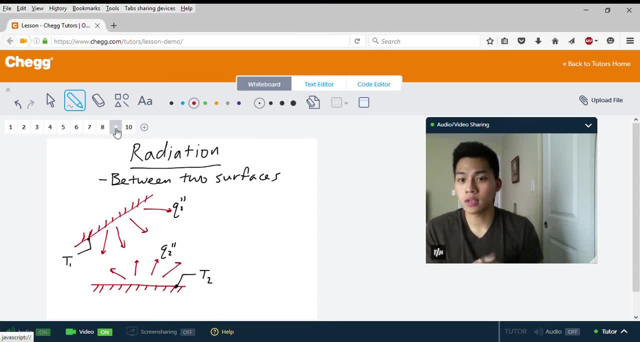 And the last mode of heat transfer is radiation, And radiation occurs between two surfaces. So, as you can see, here we have a surface up here and a surface on the bottom. This top surface has a temperature of T1, and this bottom surface has a temperature of T2.. So 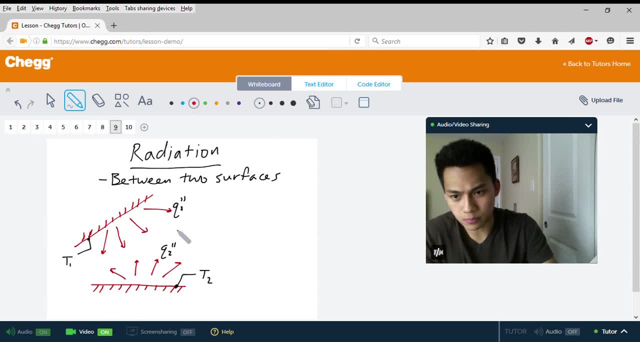 these red lines. they symbolize the heat rate. You can see we have Q1 double prime and Q2 double prime. Q1 double prime is the heat rate coming from surface 1.. Q2 double prime is the heat rate coming from surface 2.. 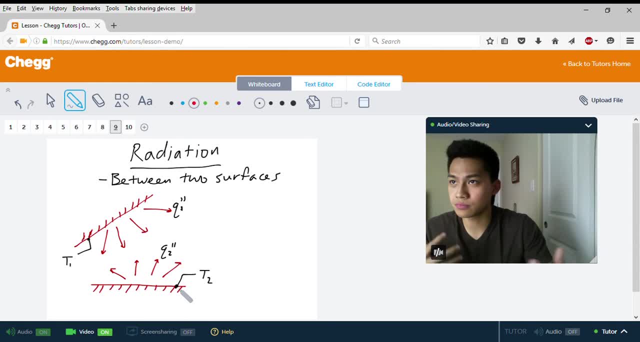 So what you can kind of imagine is: let's say we have an application of radiation would be the sun shining on Earth. We have two surfaces: the surface of the sun- Let's just draw it out just to make it more visible- We have the sun which is radiating outwards, and 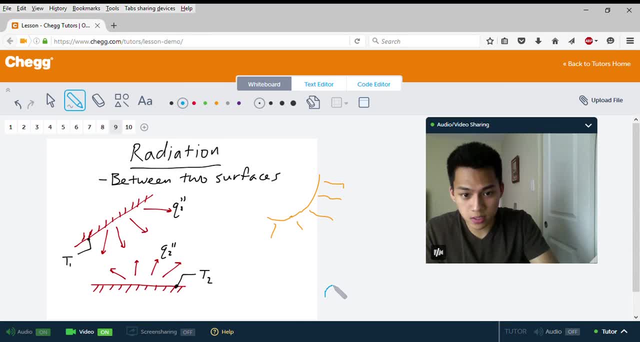 we have the Earth, however far away it is, And although it's, the Earth does have some sort of internal temperature and surface temperature, so this is also radiating outwards, So these can be considered the two surfaces and this is a perfect example of radiation We have. 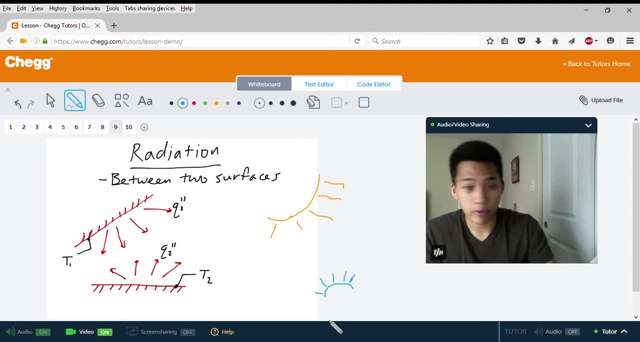 the sun, where its rays are radiating towards Earth and they essentially heat Earth. And we have the surface of Earth, which is also radiating at temperature And although it's small compared to the sun, it still is there. So we have the equation for radiation and 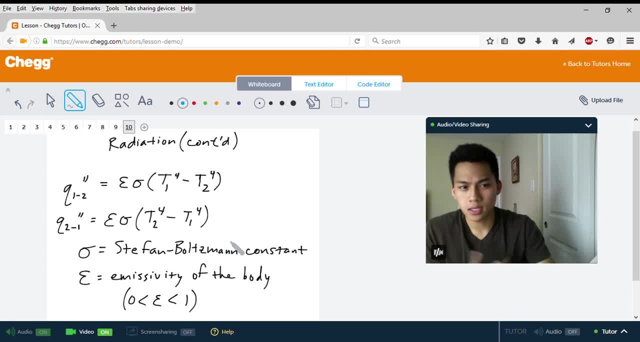 the sun is. so they're essentially different. the equation is the same, but depending on what you're applying it to, it differs. So we have Q1 and Q2.. Let me draw this sun and Earth again example. So we have the sun and Earth. Let's say Earth is surface 2, the sun 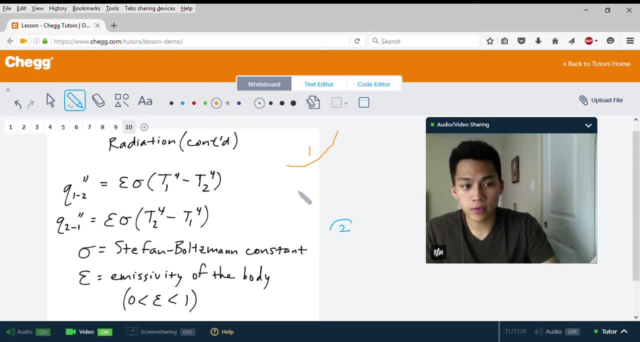 is surface 1.. So if we wanted to find the heat rate coming from surface 1 to surface 2,, which is the sun going to Earth. So if we wanted to find the heat rate coming from surface 1 to surface 2,, which is the 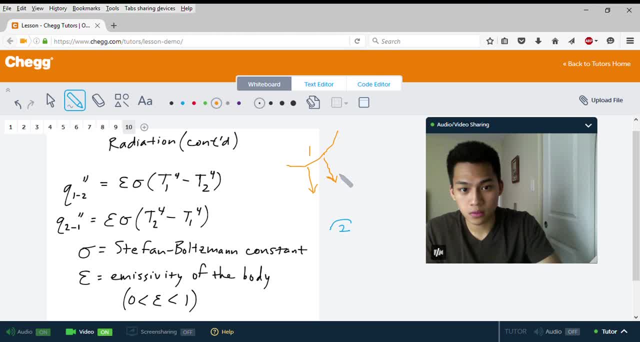 sun going to Earth, we would have the equation we have this: the emissivity of the body is what it's essentially a constant. it's between 0 and 1 times the Stefan-Boltzmann constant times T1 to the fourth, minus T2 to the fourth. 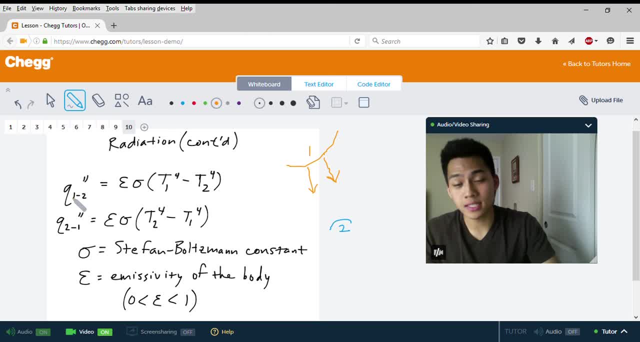 and again, if you're trying to find Q, this is the heat rate from 1 to 2. so you would use right here would be the surface temperature of the Sun to the fourth, minus the surface temperature of the Earth to the fourth. now, if you wanted to find out, 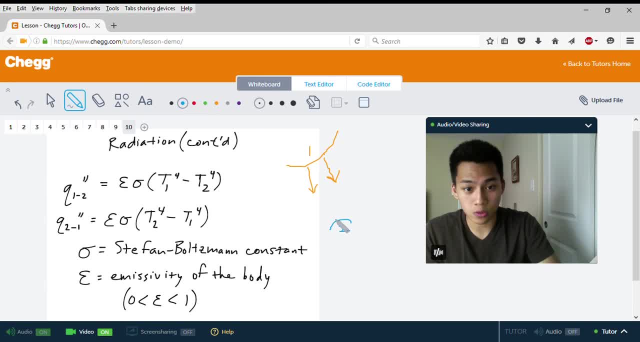 what the heat rate from the Earth is to the Sun, or surface 2 to surface 1. you would essentially just flip these temperatures right here. instead of doing T1 to the fourth minus T2 to the fourth, you do T2 to the fourth minus T1 to the fourth.